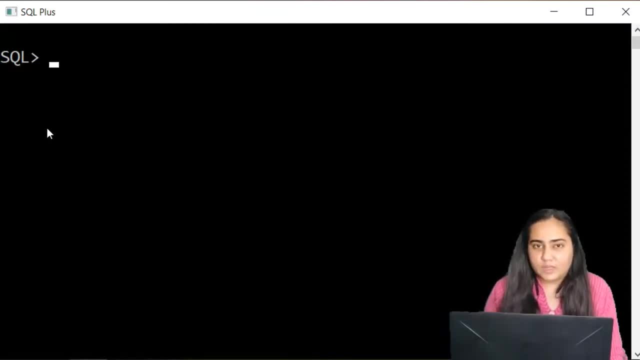 SQL plus. So if you want, you can give access to this, to your tables, to somebody else by creating an account for them. So let's do it. You can write down create user in order to create a new user, and then you'll mention the name of the user. Now suppose I want to name my user, John. 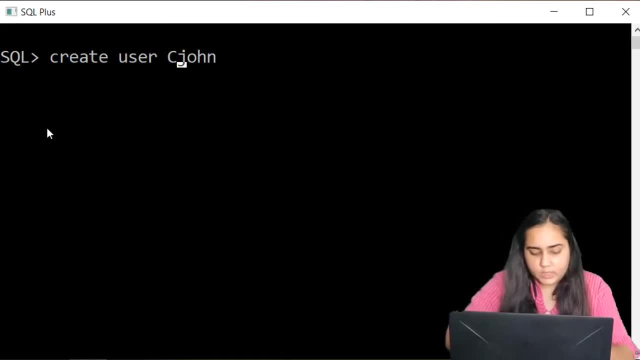 then I'm going to write before it the hash hash, because in the newest version of Oracle SQL plus you cannot name the user anything that's not starting with C hash hash. So that is necessary and I've done that, And then after that you can write down. 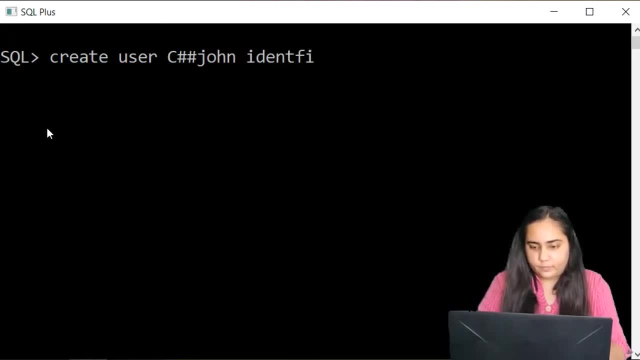 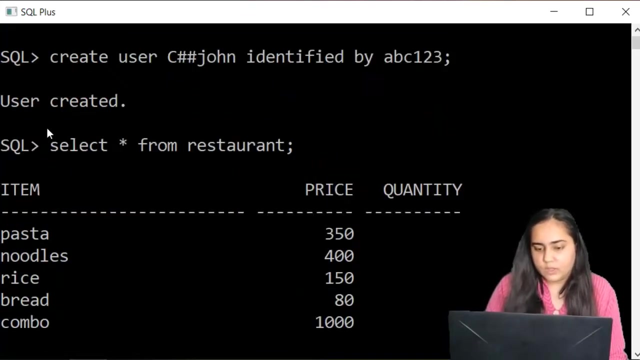 identified, identified by, and then you'll write the password. So let's just give a simple password, abc123, and put a semicolon, and then it says: create user. Now in my previous video I had created this table called restaurant, which looks like this, and right now this user cannot access this table from his or her account. Let me show that to. 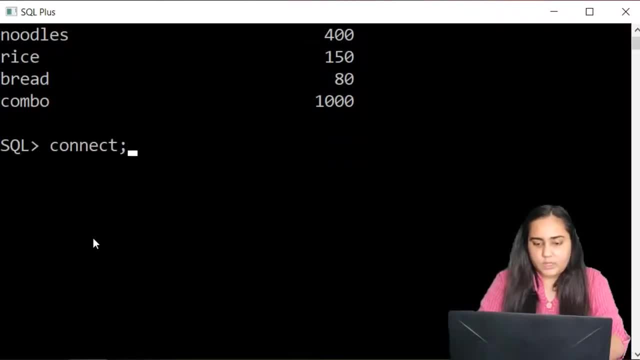 you. So I'm going to type connect, because right now I'm connected with the system account, but I want to connect with John's account. So I'll write connect And I will enter the username of John, which is c hash hash John, and the password, abc123, which you can't see but it's typed. 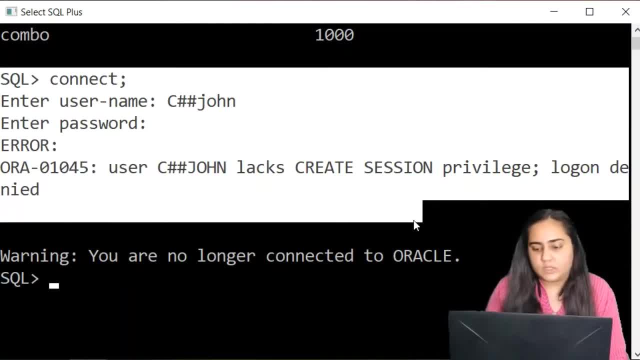 And the first error that it gives me is that John does not have a create session privilege. This means John cannot yet connect to the database until John is given the permission to connect to the database, And this permission can be given only from your system administration account. So once again you will have to. 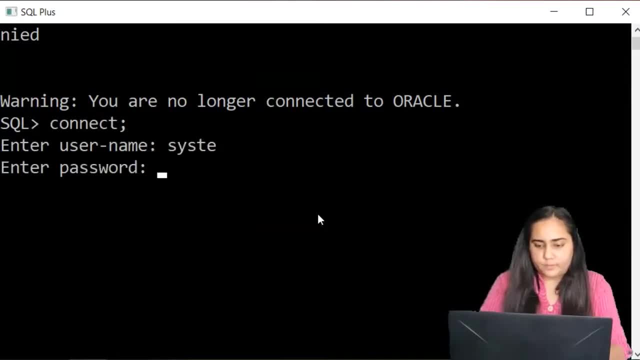 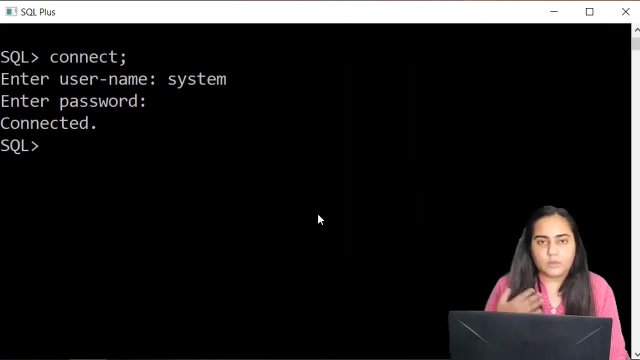 connect to your system account. Oh, I typed it wrong. that's okay. We'll connect again System and the password Once it's connected. now I'm going to give the permission to John to actually be able to log hello into my system Every. 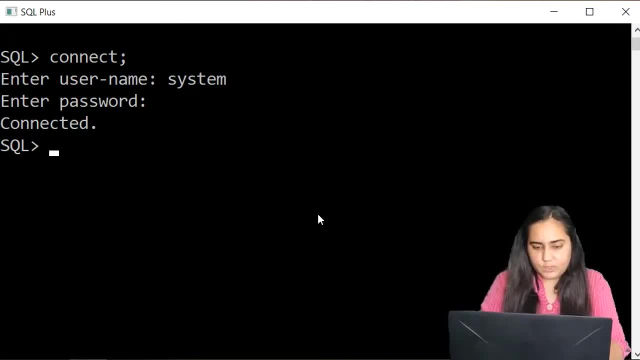 to log into the system. so I'm going to write here grant. grant is the command to give permission. so grant create session. create session means allow John to log in. grant create session. to see hash, hash, John and semicolon and it says grant succeeded. now let's see if John can connect or not. so let's type username. 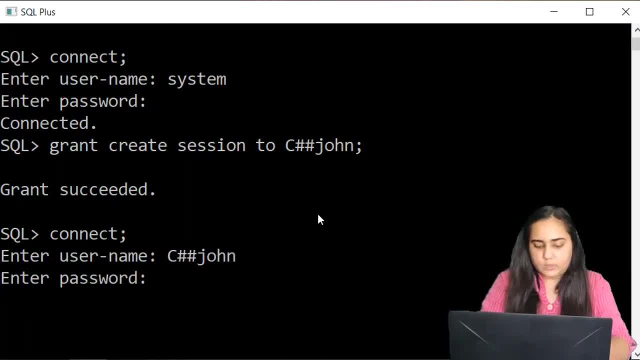 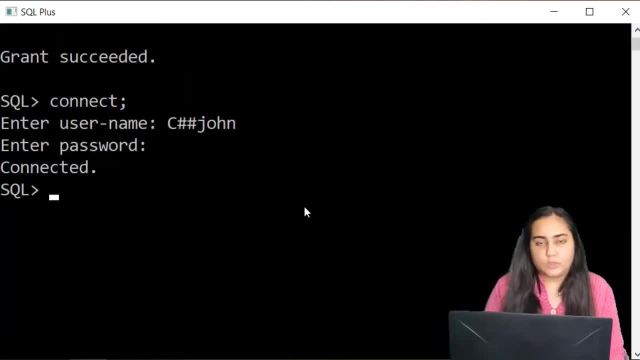 John password ABC, one, two, three and it says connected. so now John is able to connect and John can create tables and John can view his own tables. but John cannot view your tables. yet the tables created by his own tables are not connected to his own tables, so that's. 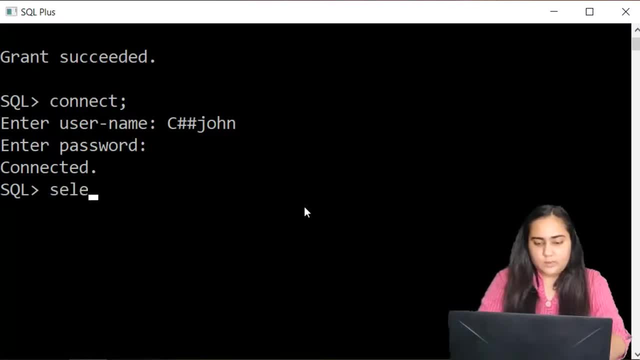 by you from your system account. Let us see if I do select tar from now. in order to access a table that is created by system, I need to write systemname of the table. So the table is restaurant and you will see. it says table or view does not exist. 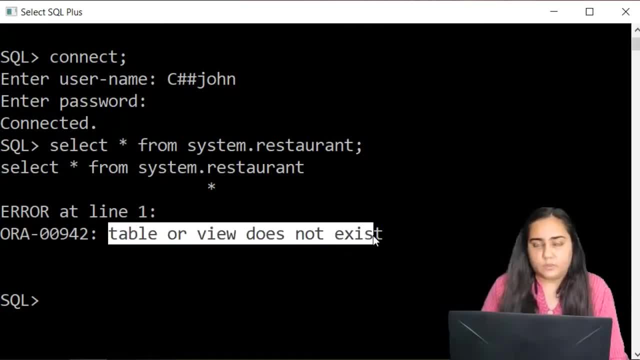 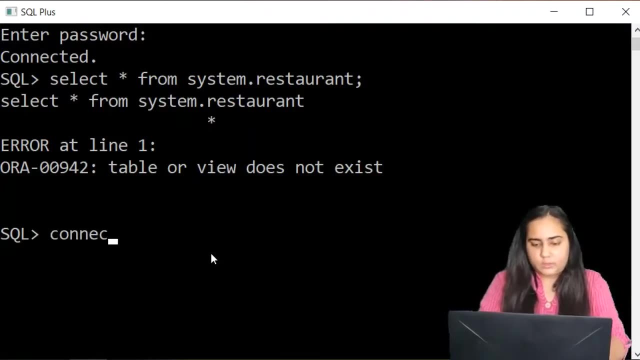 It actually exists, but John won't be able to see it because John does not have the right to be able to access this table. So let's connect from system and give this right to John. So once again, connect and I'm going to type username. 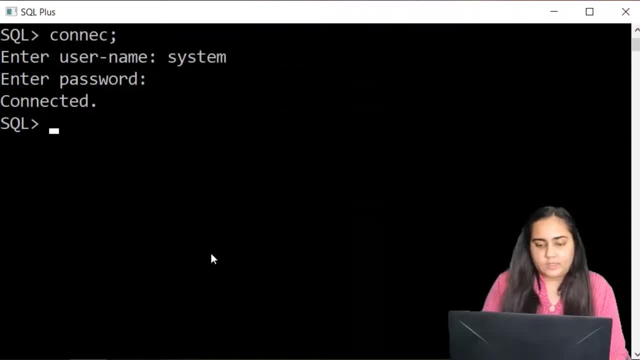 password and it says connected. Now I'm going to grant the right to select on my table, And let's say that I also want to allow John to insert new values. Then I'm going to write grant select comma insert on and I'll specify the name of the table. 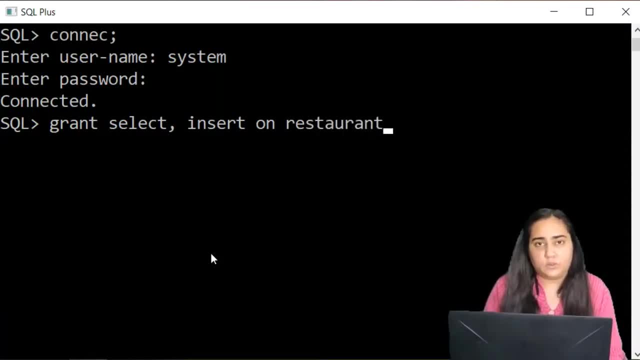 because I don't want to give right to select and insert into all tables that I've created. I just want to give this a permission on restaurant table. So on restaurant, and then you'll write to C hash hash, name of table, and then utis and 13 and Gmail pos. 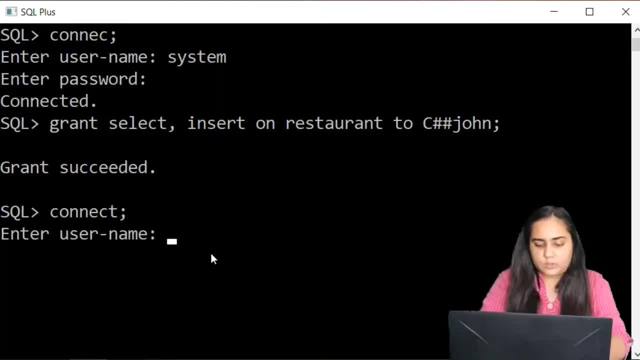 Againрут check D. So without using the Jamf Alt mode, I already typed this into my odd table And so now I'm looking at the table node. So I don't want to actually create a new table. I'm going to type in: 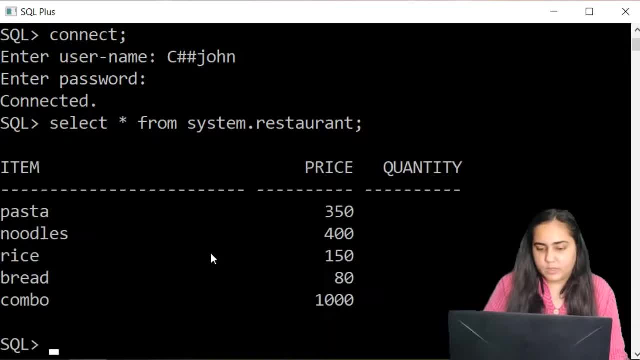 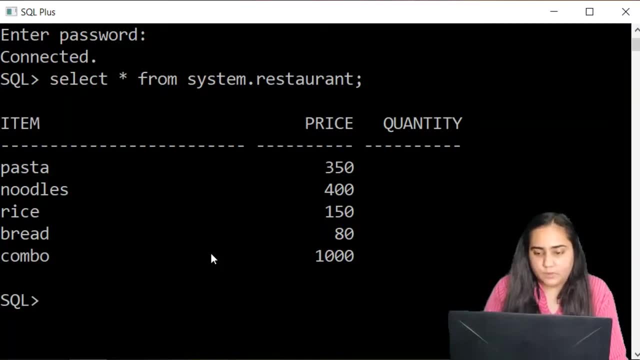 restaurant and we'll put a semicolon and you can see that John can now actually access the table and view the, the entire table as it is now. let's see if John can insert something into this table. so insert into restaurant values and let's say I want to insert some item. let's insert ice cream and let's insert a. 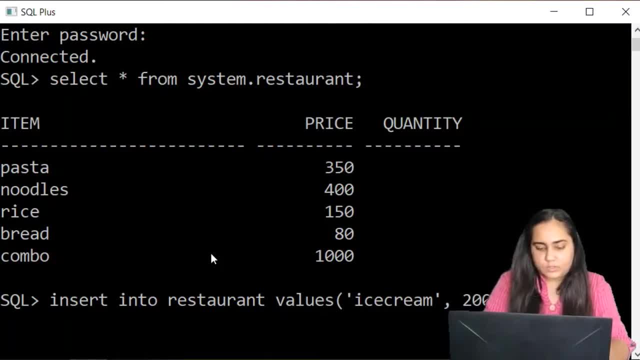 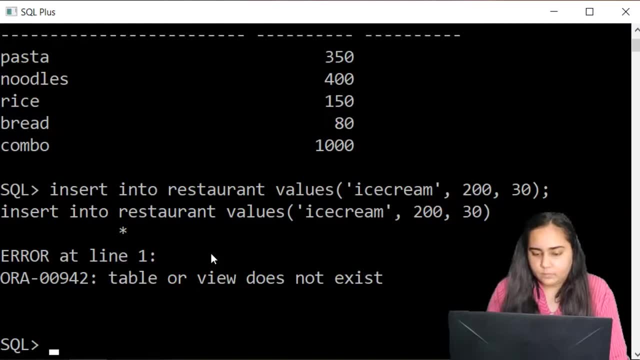 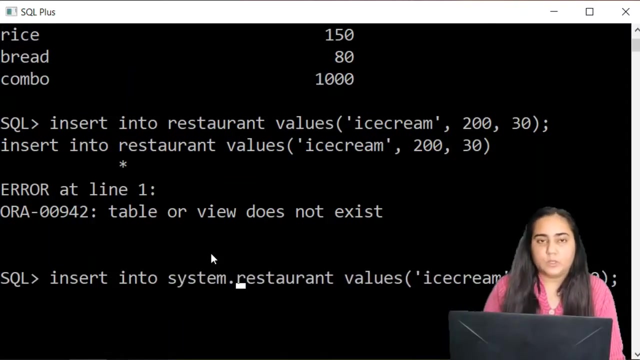 price 200 and quantity 30 and semicolon enter. now it gives me an error that table of you does not exist because I forgot to mention that this is. table of you does not exist because I forgot to mention that this is system dot restaurant. we'll see when I'm typing just restaurant, that means 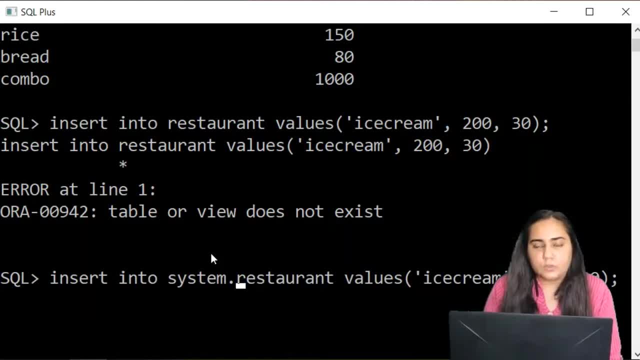 I'm trying to insert something into a restaurant table created by John, but John hasn't created any tables. so if you want to insert into systems table you need to write system dot restaurant. so once that is done you can hit enter. it says one row created, so let's take a look at it. select start. 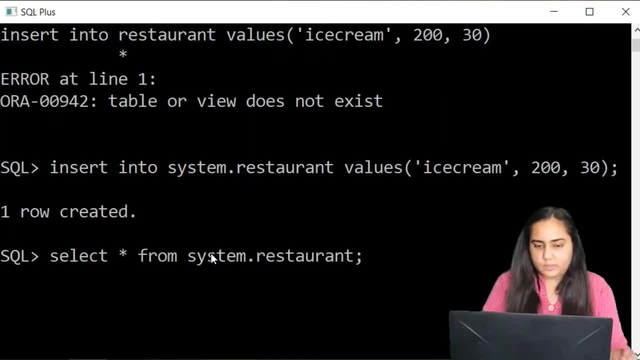 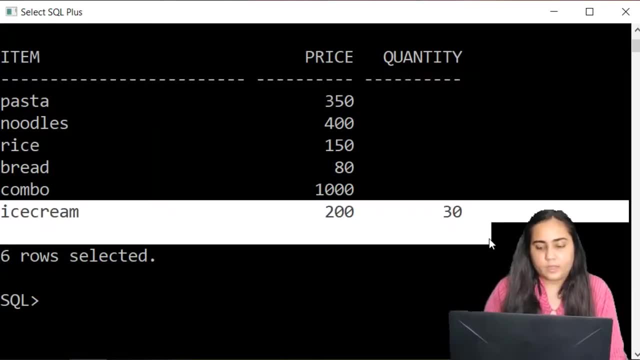 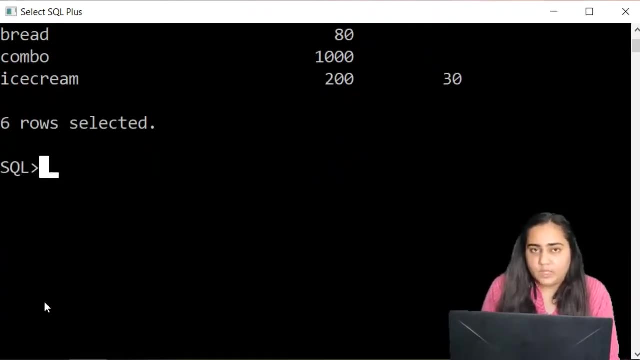 from system dot restaurant and you can see that row has been added inside. now let's see if I can delete something from here because, if you remember, I have only given John the permission to perform, select and insert on the restaurant table, but not update and delete. so we need to check if John can update and 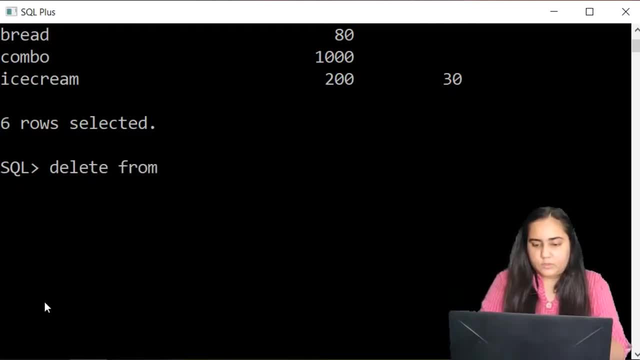 delete. so let's say that John wants to delete something, so I'm going to delete from restaurant. let's try to delete everything where the price is, where price is greater than hundred. so and once again you need to type system dot restaurant, not just restaurant, and let's hit enter. 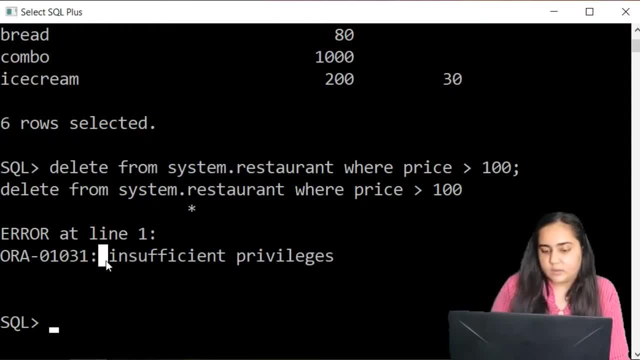 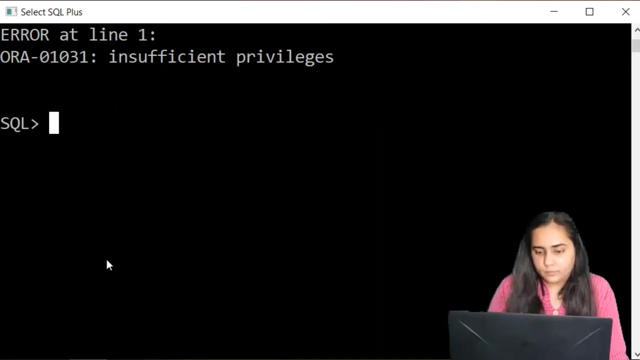 and you can see, it gives me an error this time that says insufficient privileges, because I do not have the permission to delete anything from here. I can, however, select and insert. I cannot delete and update because no permission. now let's go back to the system. let's go back to the system account that we have. 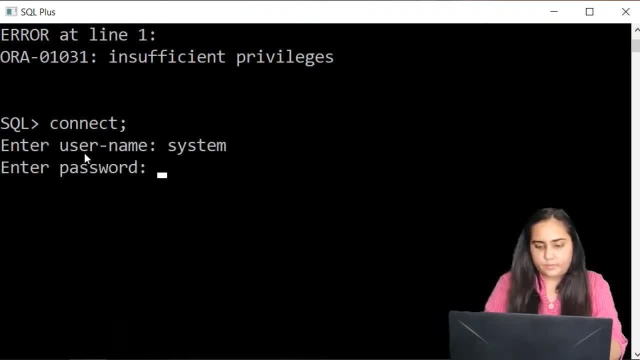 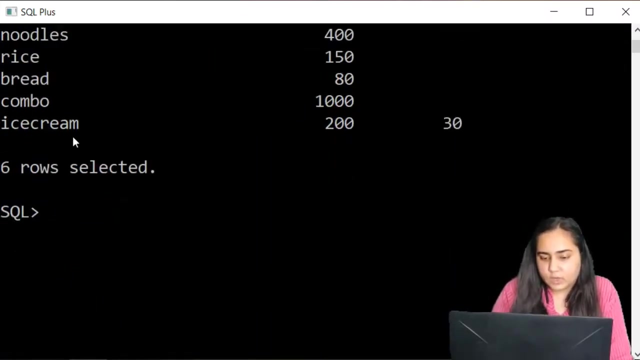 so let's connect to it and let's check what the table restaurant looks like now, because restaurant was created from system. you just need to write select star, not estiux Soldier, anything from there. you can see here how ice cream has been added, which was added by John, but you can view it from here to to show that it is. 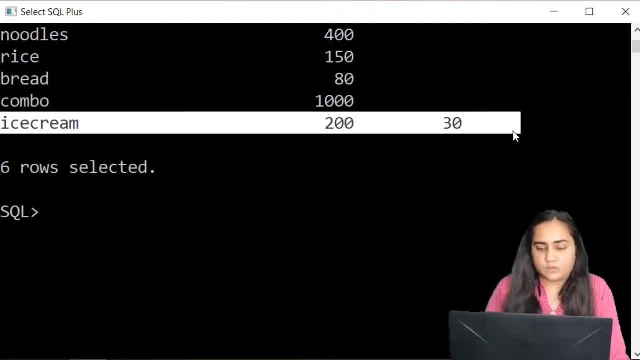 created and blanked it. if you fill the blank, check this stitch ginger, find it here that it's not actually a copy that John is accessing. John is able to access the same table And let me just show you how you can also provide update and delete to John. 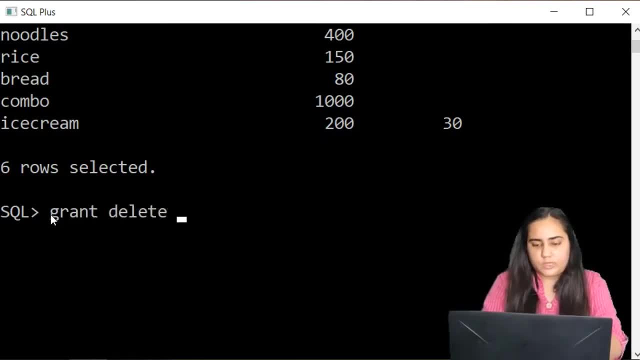 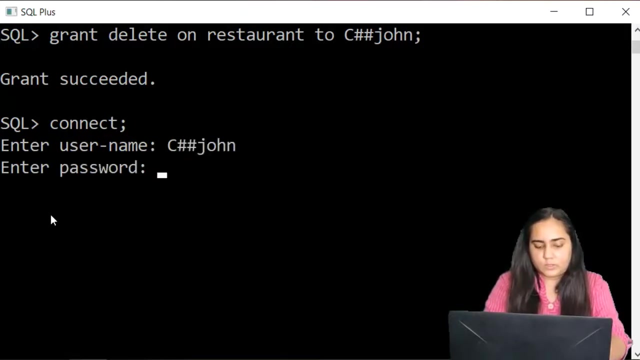 So let's just grant one more write to John to delete on restaurant to C hash hash John And it says grant succeeded. So once again I'm going to go back and connect to John's account. It was C hash hash John, Password is abc123, says connected. 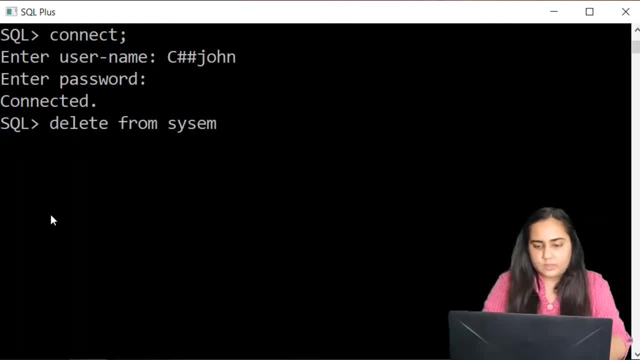 This time I'm going to do delete from systemrestaurant where rise greater than, let's say, 400.. And let's press enter And it says one row deleted. Let's check which one. So select star from systemrestaurant And yes, the combo row is gone. 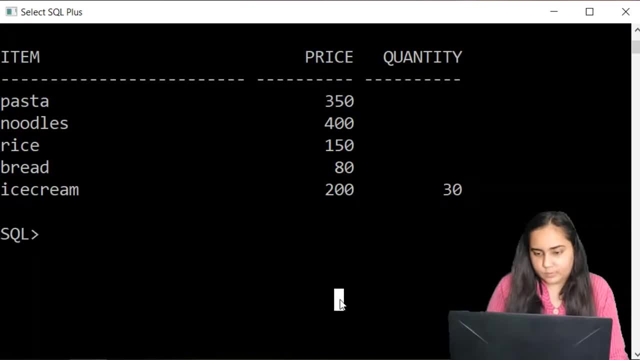 which was having a price of 1000.. So John can now perform deletions, but can John perform optations? He cannot, because we haven't given him the right to update anything. For example, if John tries to do systemrestaurant set price. 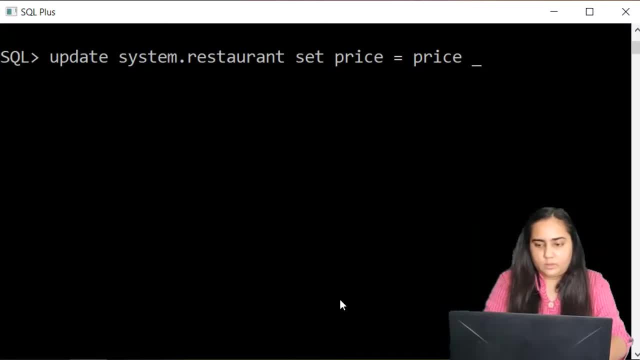 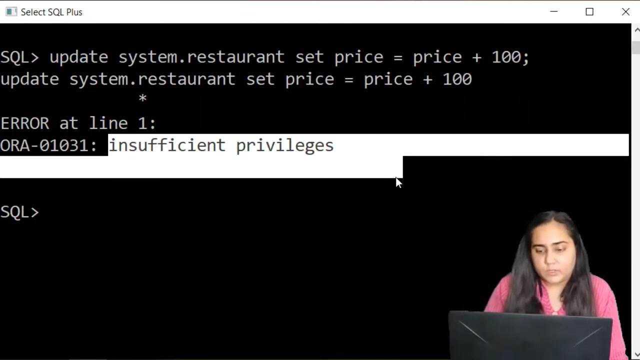 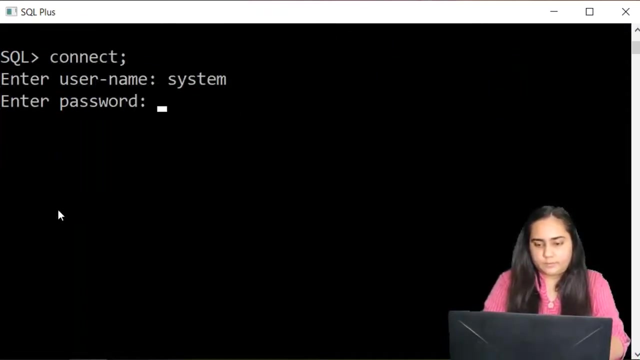 let's say he wants to increase the price of everything by 100, then it's going to give the error that the privileges are insufficient, which means John does not have the privilege to do this. Now let's go back to the system account and take away the permission from John. 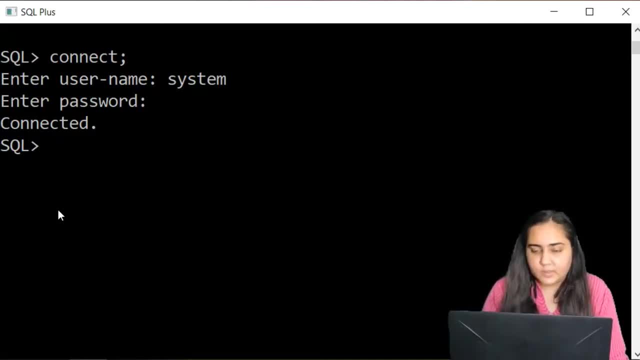 So remember how I allowed John to delete something from the table. Now I don't want to allow John to delete something from the table. Then I'm going to write: revoke, delete on the table restaurant from the user John. from the user John. from the user John. 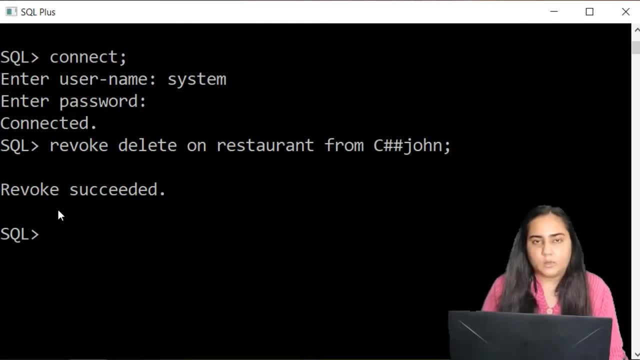 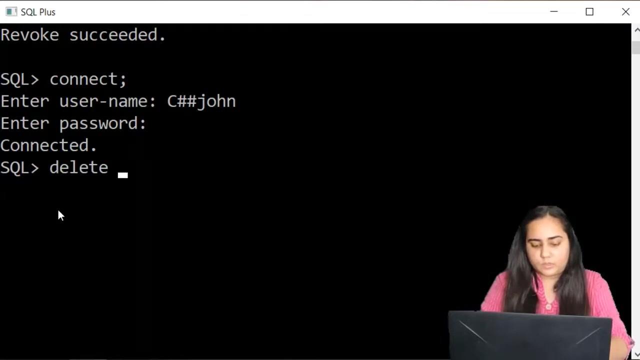 And it says: revoke succeeded. And once again you know what we are going to do. now Connect to John's account and enter the password And now try to delete something from the restaurant table. So delete from system dot restaurantrestaurant where- and I'm going to pass something- where price is greater than, say, 200 and semicolon.